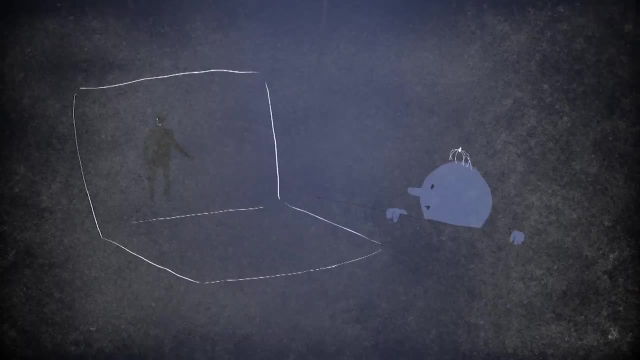 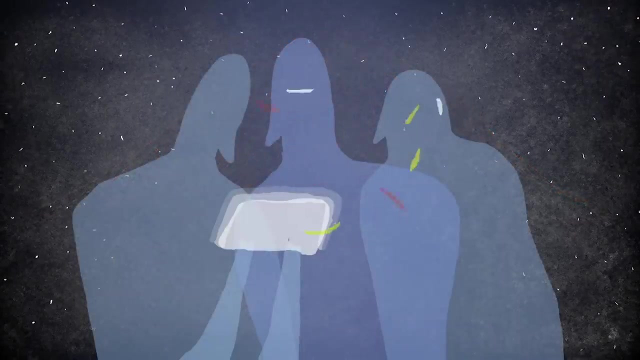 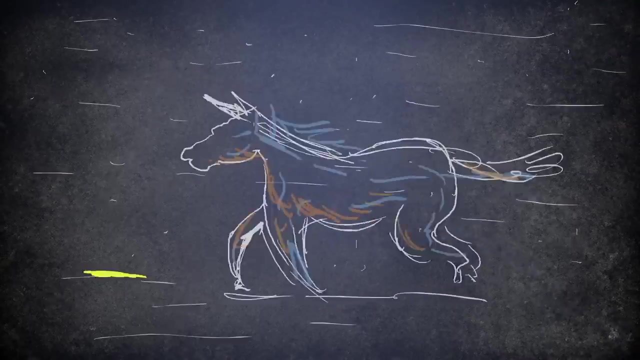 amplifying the impact of speakers. What is more, we can enhance these skills in ways that agents could never have imagined: the ability to show right there, in beautiful, high resolution, any image that a human can photograph or imagine. the ability to weave in video and music. 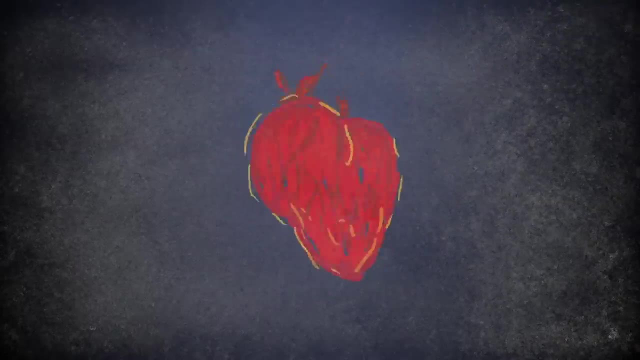 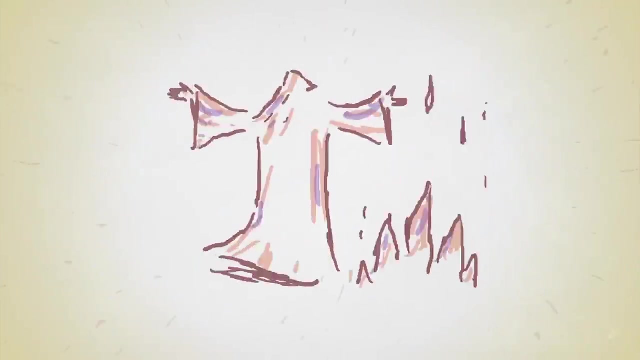 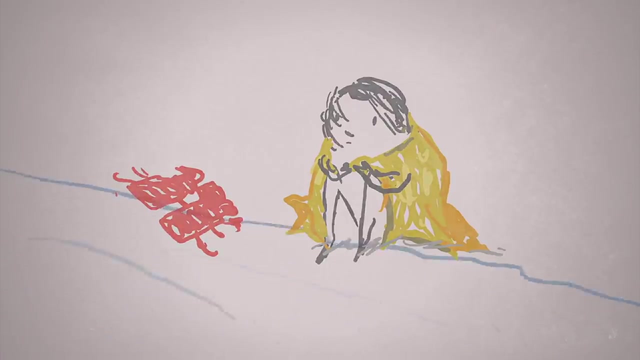 the ability to draw on research tools that present the entire body of human knowledge to anyone in reach of a smartphone. suddenly, an ancient art has global reach. we need that now more than ever. ideas that could solve our toughest problems often remain invisible because the brilliant people in whose minds they reside lack the confidence or the know-how to share those. 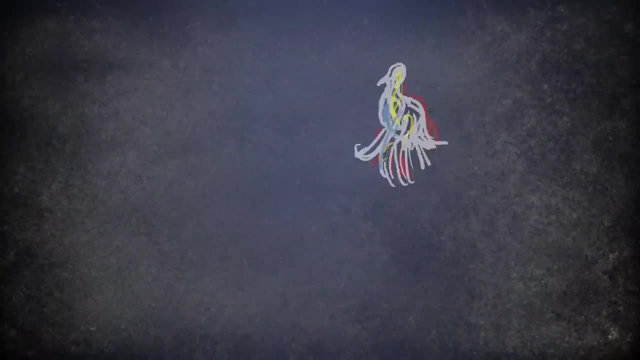 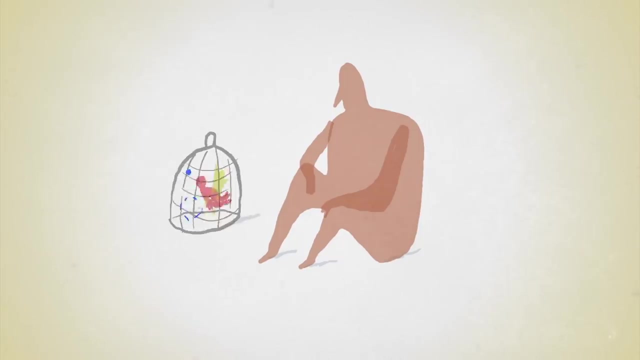 ideas effectively. at a time when the right idea, presented the right way, can ripple across the world at the speed of light, there's huge benefit to figuring out how best to set it on its way, both for you, the speaker in waiting, and for the rest of us who need to know what you have to say. 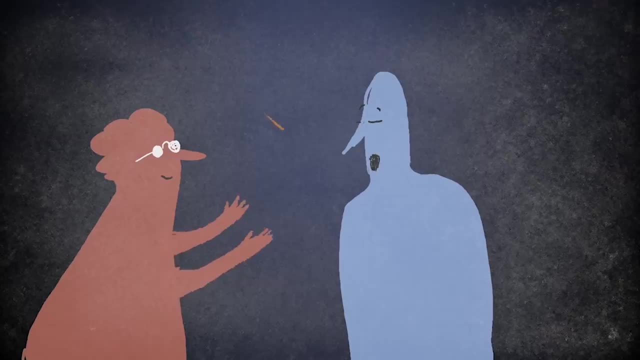 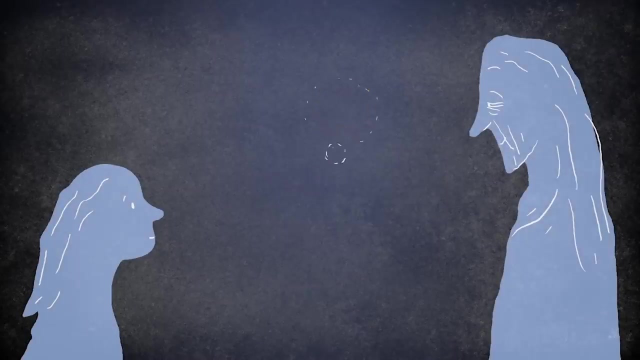 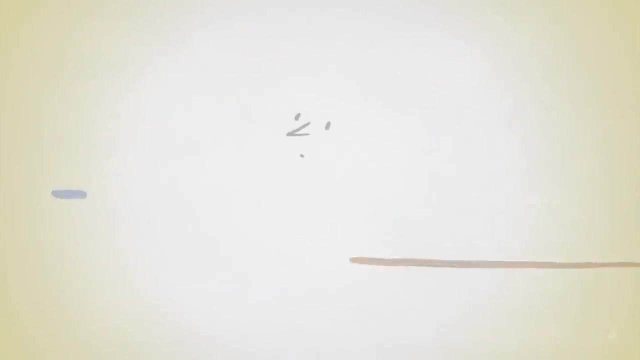 the good news is, these skills are teachable. they absolutely are, and that means that there is a new superpower that anyone, young or old, can benefit from. it's called presentation literacy. i've become convinced that tomorrow, even more than today, learning to present your ideas to other humans will prove to be an 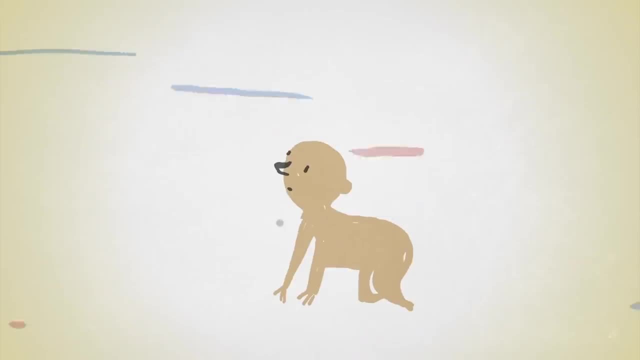 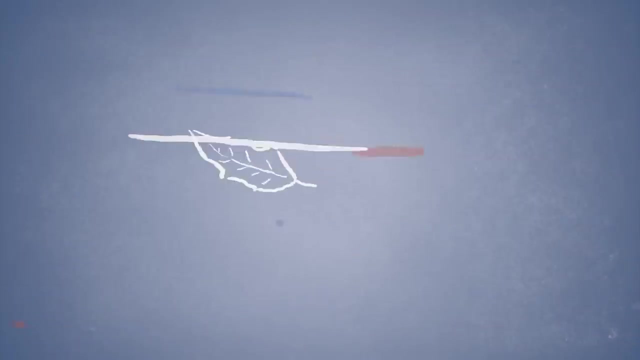 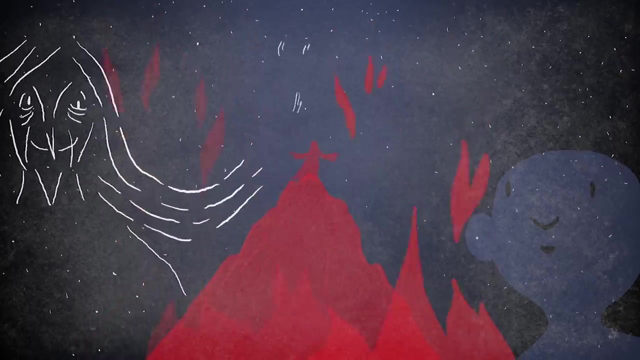 absolutely essential skill for any child who wants to build confidence, anyone who wants to progress at work, anyone who wants to leave a legacy, anyone period. the campfires of old have spawned a new kind of fire, a fire that spreads from mind to mind, screen to screen, the ignition of ideas whose time has come. 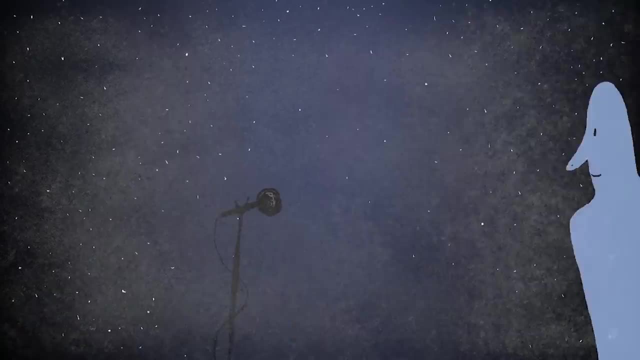 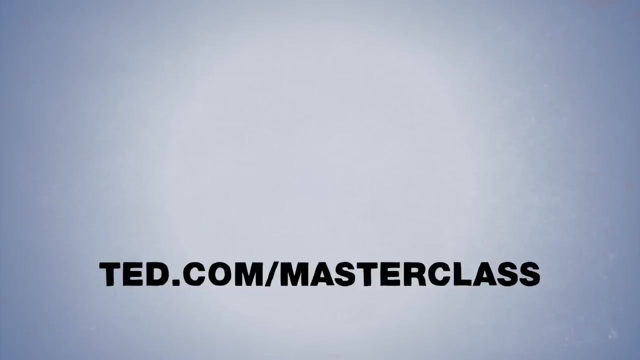 this matters. let's go light a fire. if you're ready to find and share your spark, we have an app for you. download ted masterclass, ted's official guide to public speaking, and try lesson one for free today. be a part of a grand and ancient tradition and discover your ideas worth sharing.